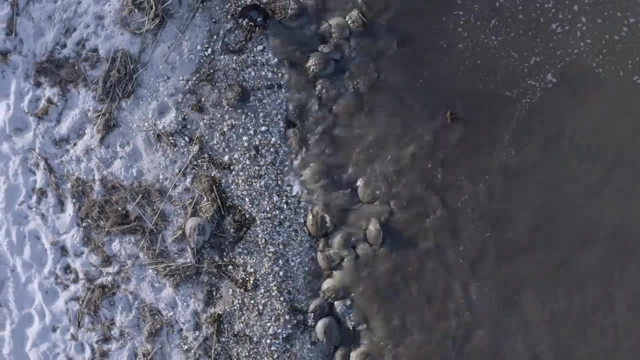 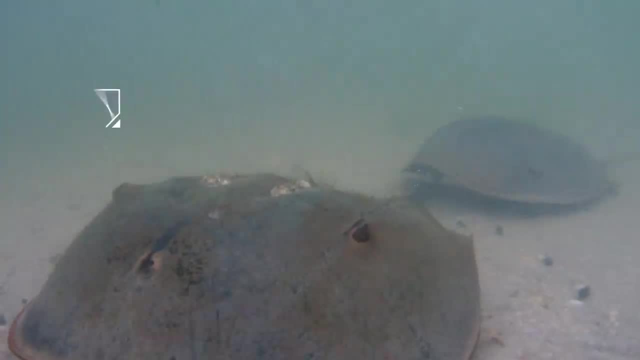 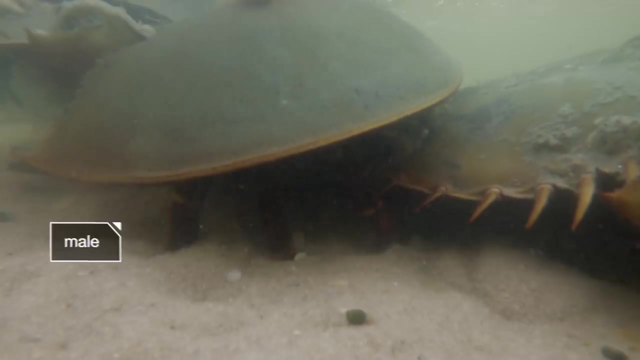 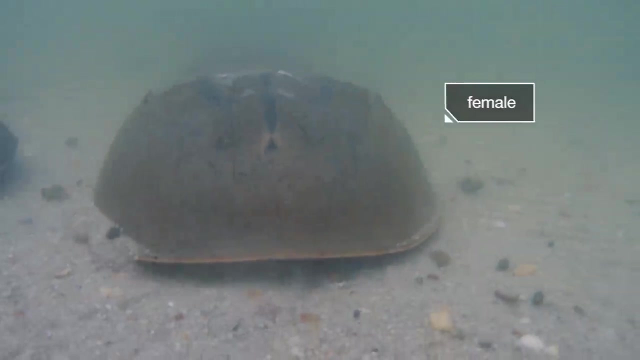 some of the biggest. The males show up first, hanging out on the beach and in the shallows of the bay. They scramble to latch onto the backs of passing females. The females can be the size of dinner plates, way bigger than the males. 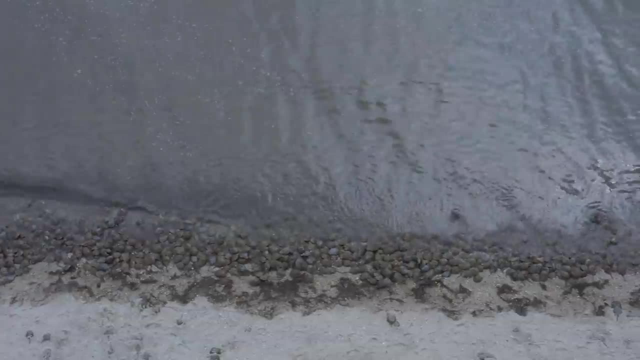 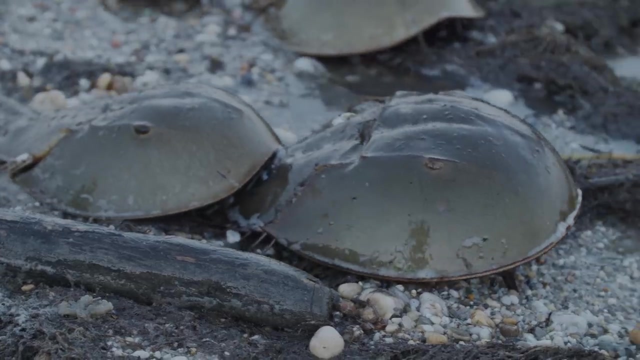 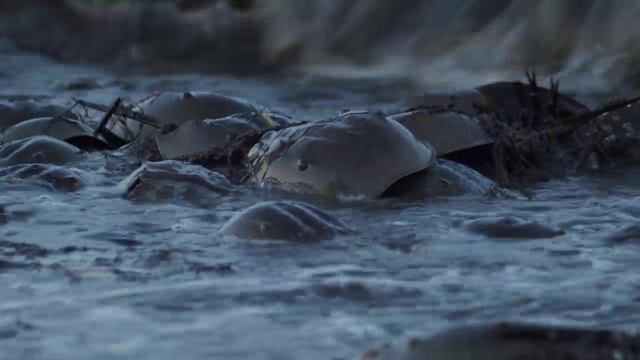 Success. They take advantage of the fleeting high tides to haul their precious cargo as high up the beach as possible. The females muscle their way up the beach with the males in tow. The greatest danger for these horseshoe crabs is flipping over. 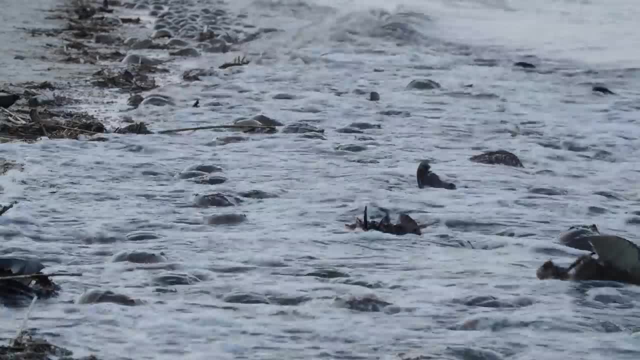 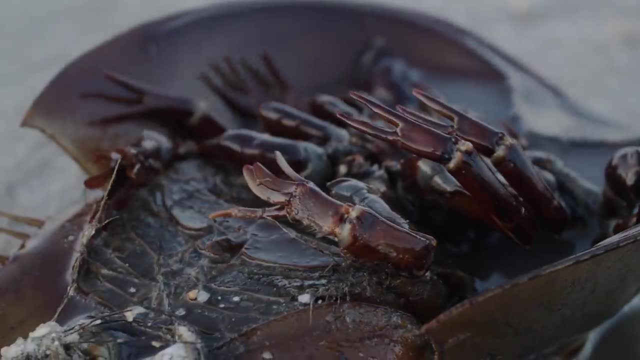 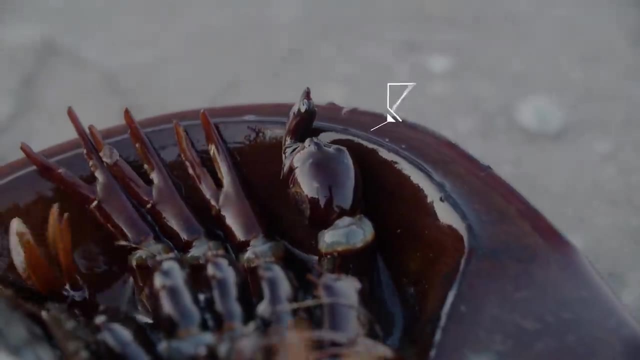 Exposing their vulnerable underside, And it only takes a small wave to do it. Under the hood. horseshoe crabs' legs end in pincers, But mature males have something special on their front legs: This clasper that looks like a little boxing glove with a hooked finger. It's perfect. 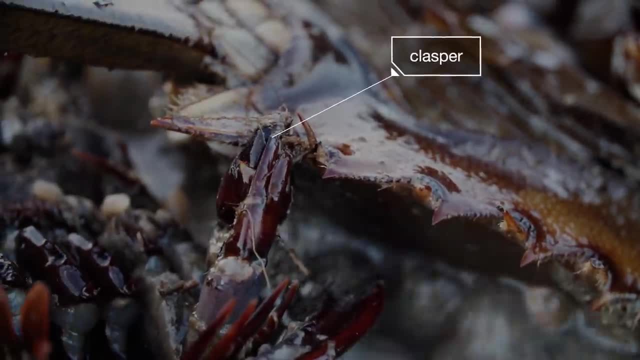 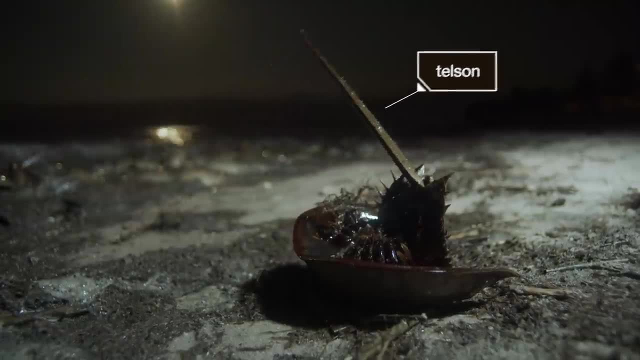 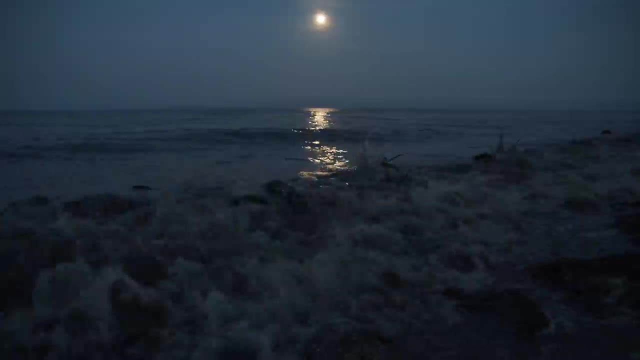 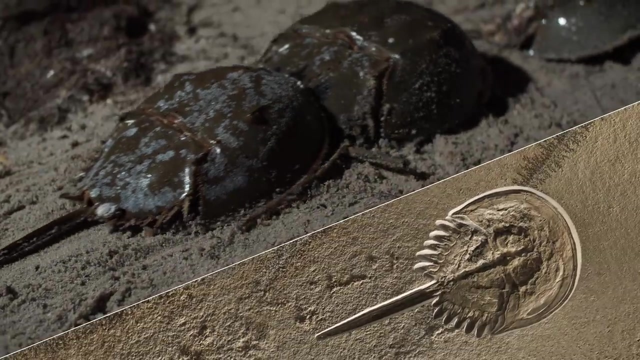 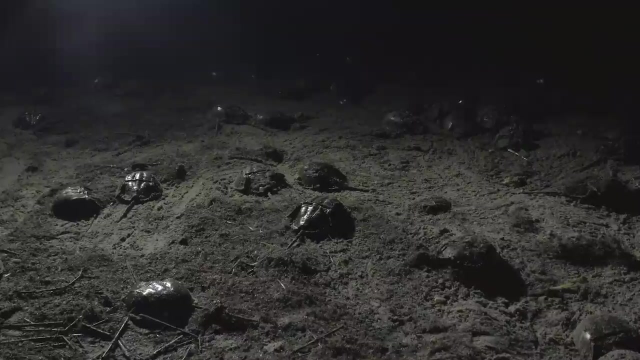 Horseshoe crabs have been making these high tide treks under the glow of the full moon since before the dinosaurs, That's more than 400 million years ago. Not everyone finds a date, Especially those younger males, But they hike up the beach anyway. 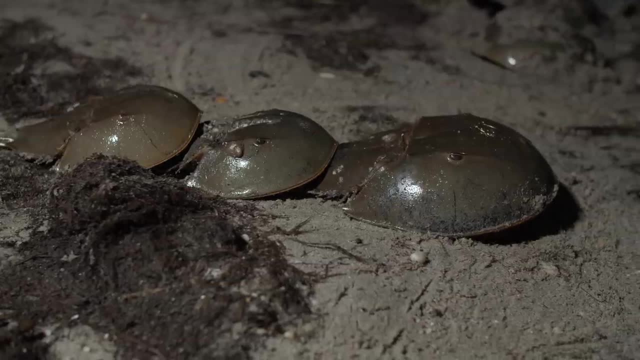 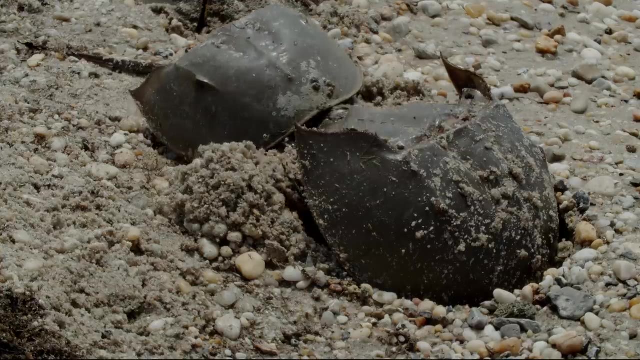 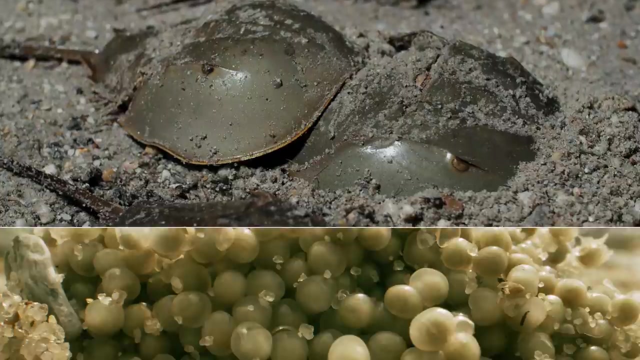 in hopes of getting in on the action. This female is dragging around two admirers. When a female finds a good spot, she digs and digs into the wet sand. The female lays roughly 4,000 eggs in one go. The male that clung to her all this time.